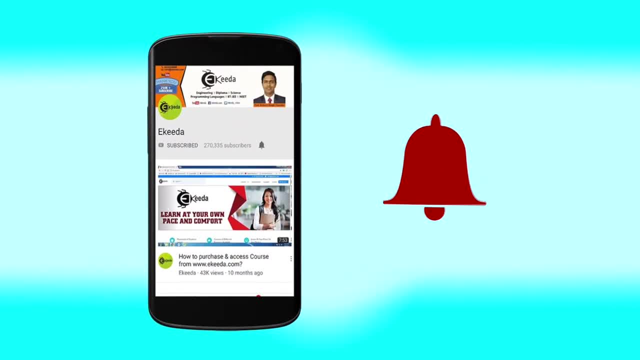 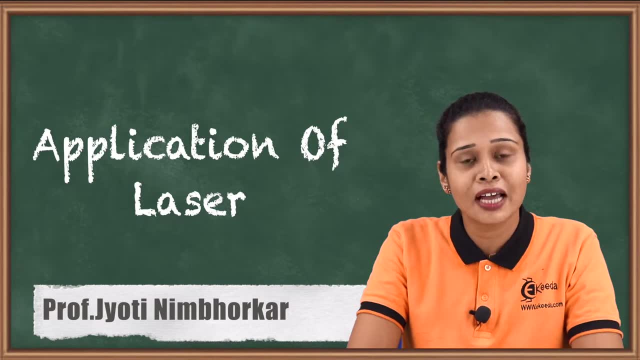 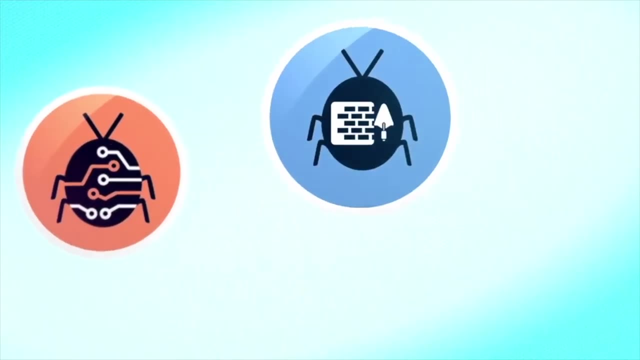 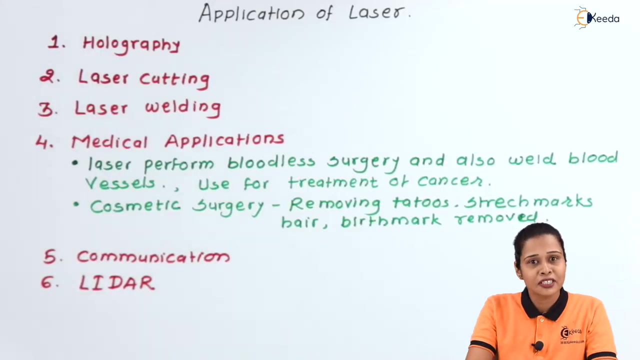 Click the bell icon to get latest videos from eKIDA. Hello friends, today we will see application of laser. Laser are used in the medical field as well as in industry purposes also. So let us see briefly what are the applications. The first application of laser is a holography. Holography is a technique in which we are getting 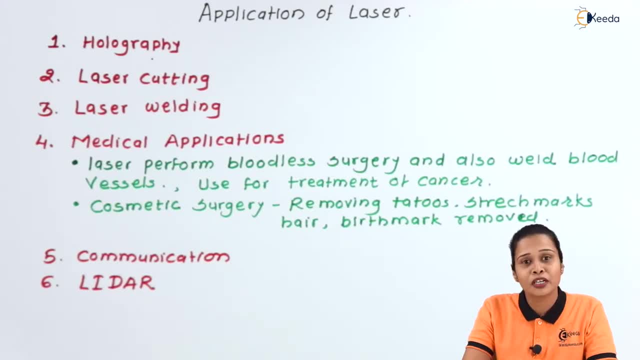 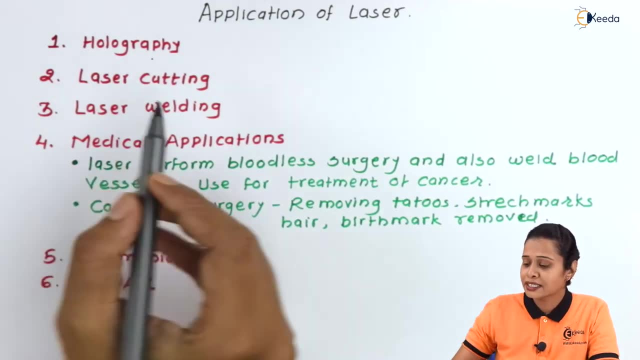 3D image of the 3D object, which is very important to study the molecular structure and the crystalline shapes. Next application is laser cutting. Laser cutting is used in the garment industry. Laser cutting is used in the garment industry. Laser cutting is used in the. 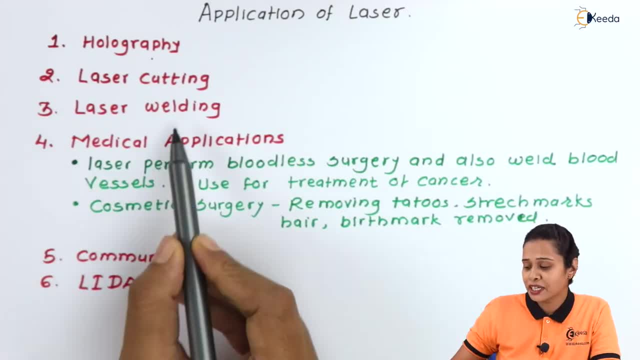 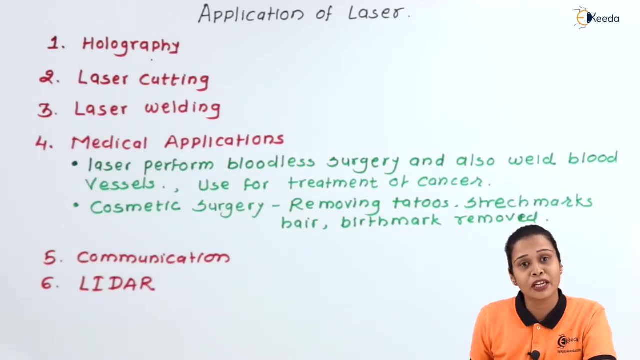 to cut the garments. Then next application we have that is laser welding. Laser welding is a technique in which we can join multiple pieces of the metal by using the laser. Then there are so many applications. that is a medical applications. Laser perform bloodless surgery and it also weld. 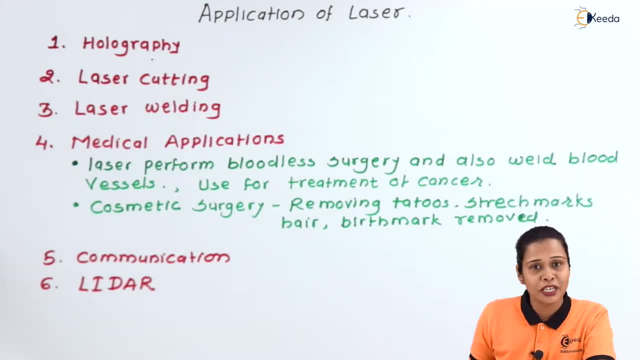 the blood vessels. It is used for the treatment of cancer. Then in cosmetic surgery also, laser plays a very important role in the treatment of cancer. So laser cutting is used in the important role, For example, removing of tattoos, stretch mark, hair and birthmark removal. So all 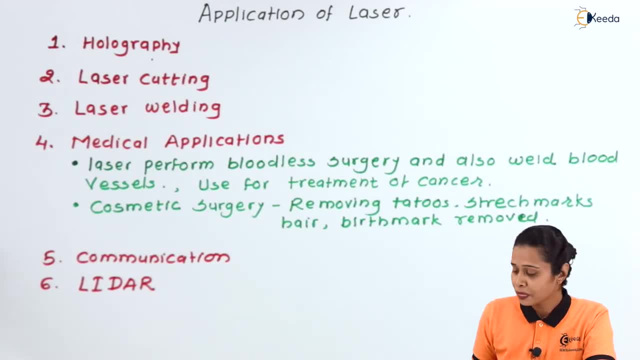 this surgery can be happened with the help of laser. Then we have a communication. In optical communication system, laser plays a very important role. Then we have lidar. Lidar is light detection and ranging. It is used to find the distances between the object. For example, we have one. 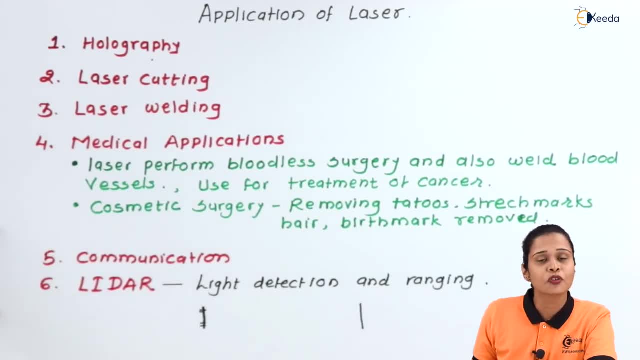 object here and, for example, we have a laser, So we have a laser, So we have a laser, So we have other thing is here, So if you want to find out the distance between this object, So we will send.